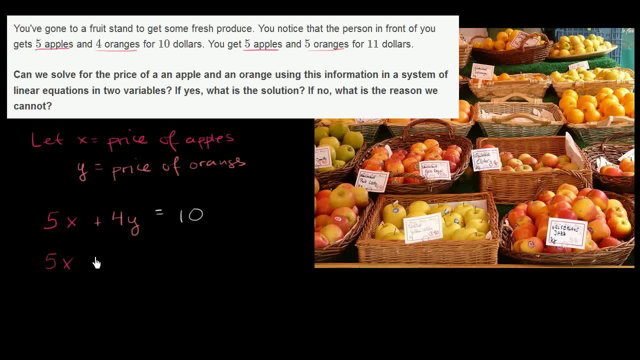 And then you buy five oranges. So you're going to pay five oranges times the price per orange, Which is y. So this is how much you spent on oranges. This is how much you spent on apples and oranges. this sum And they tell us that this is going to be $11. 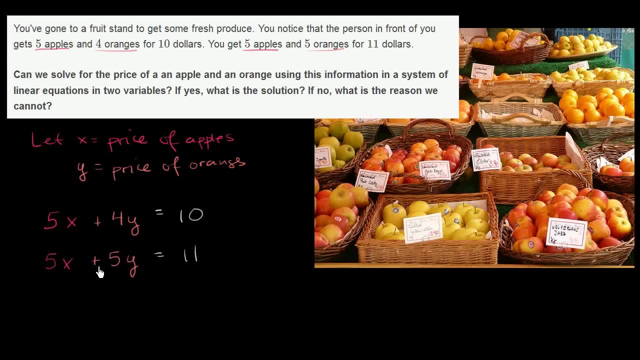 So can we solve for an x and a y? And it looks like we can. And a big giveaway right over here is: the ratio between the x's and the y's in these two equations are different, So we're getting some information here. 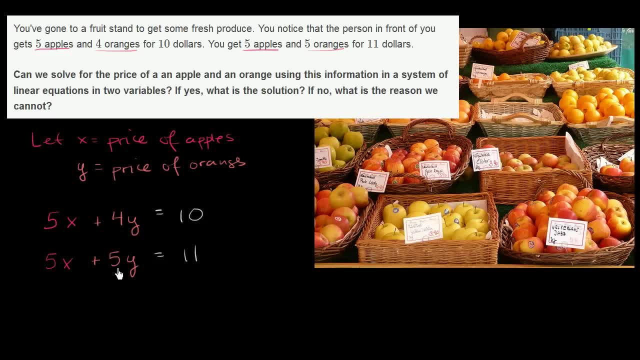 If the ratios were exactly the same, if this was 5x plus 4y right over here and we got a different number, then we would be in trouble Because we bought the same combination but we got a different price. But the good thing is that we have a different combination. 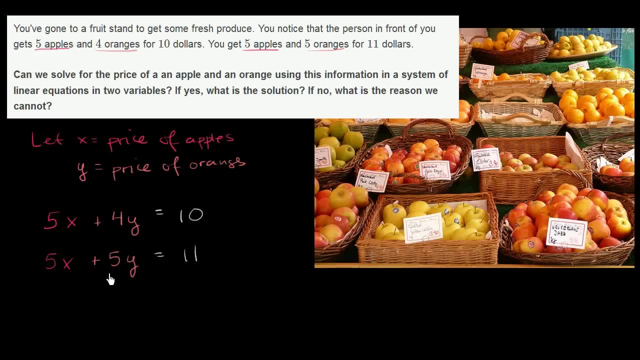 here. So let's see if we can work it out Now. the most obvious thing that jumps out at me is that I have a 5x here and I have a 5x right over here. So if I could subtract this 5x from that 5x, 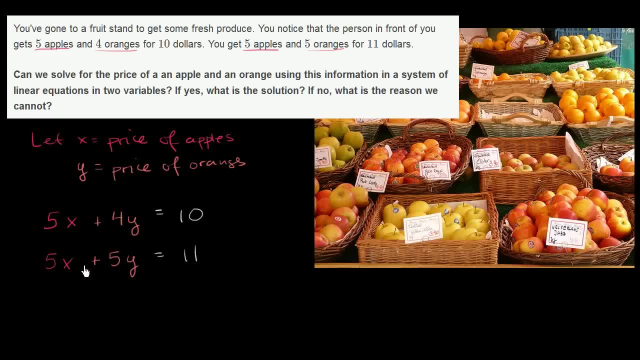 then I would cancel out all of the x terms. So what I'm going to do is I'm going to multiply this bottom equation by negative 1.. So it becomes negative 5x minus 5 or plus negative 5y is equal to negative 11.. 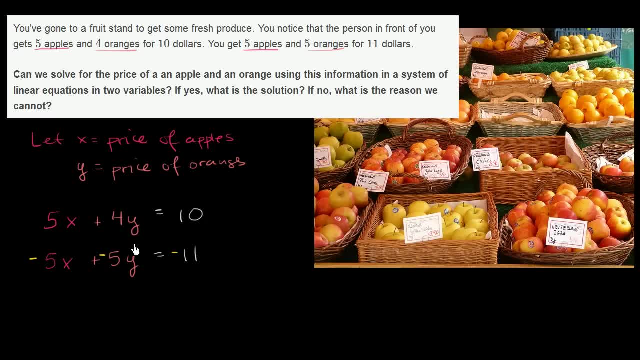 And then I'm going to. So I'm going to essentially add both of these equations, And I can do that because I'm doing the same thing to both sides. I already know that this thing is equal to this thing, So I'm just adding those things to either side. 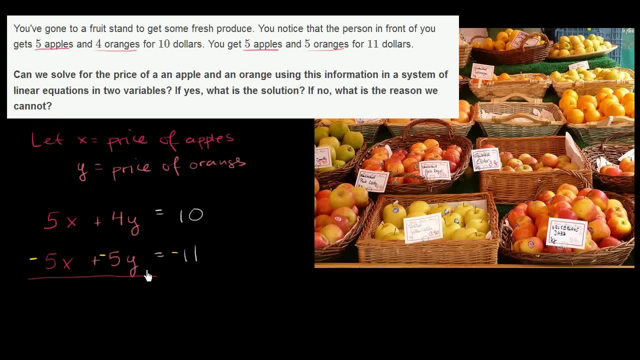 So on the left-hand side, I have 5x minus 5x- Well, those cancel out. And then I have 4y minus 5y- Well, that's negative y, And that's going to be equal to 10 minus 11, which is negative 1.. 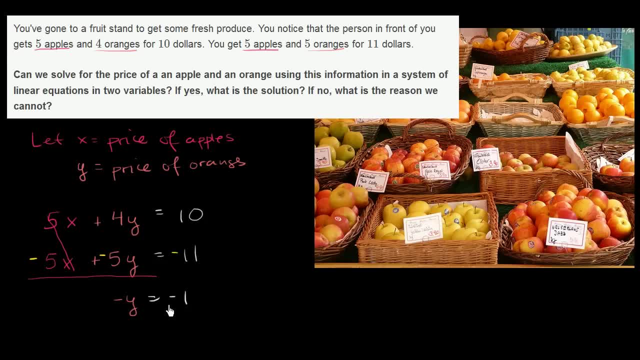 And then if we multiply- If we multiply both sides of this times negative 1, or divide both sides by negative 1, we're going to get y is equal to 1.. So, just like that, we were able to figure out the price of oranges. 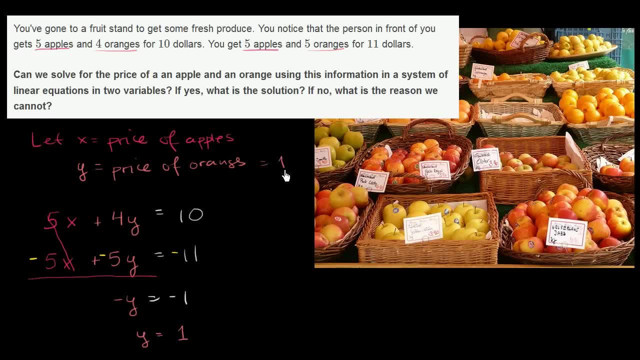 It's $1 per orange. Now let's figure out. So this is equal to 1.. Now let's figure out the price of apples. So we can go back into either one of these equations. I'll go back into this first one. 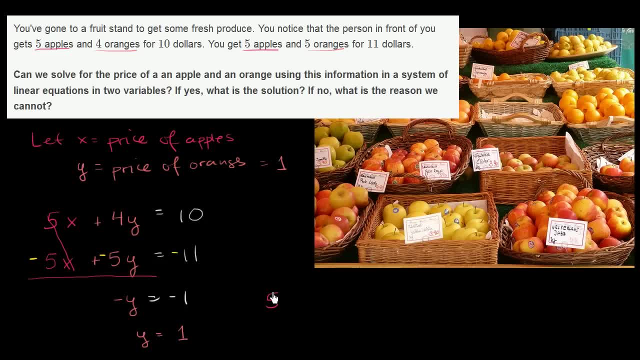 So let's go to the person in line in front of us. They bought five apples at x dollars per apple, plus four oranges at $1 per orange, And they spent a total of $10.. They spent a total of $10. So this, of course, is just 4.. 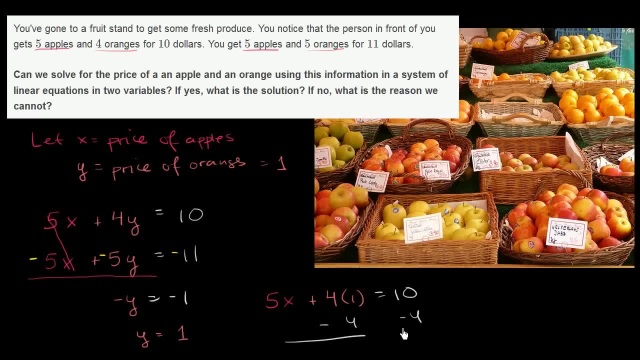 Let's subtract 4 from both sides And we get, well, 4 times 1 minus 4, that just cancels out. We're just going to be left with 5x on the left-hand side. We're just going to have 5x on the left-hand side. 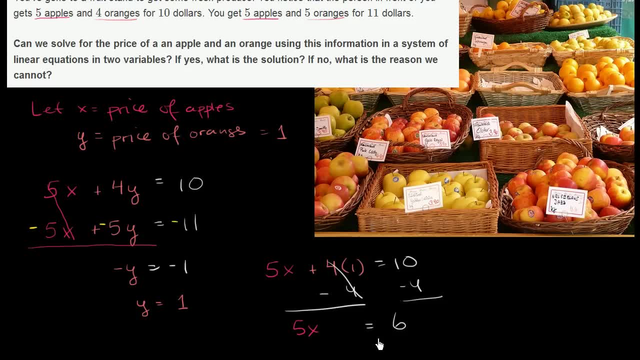 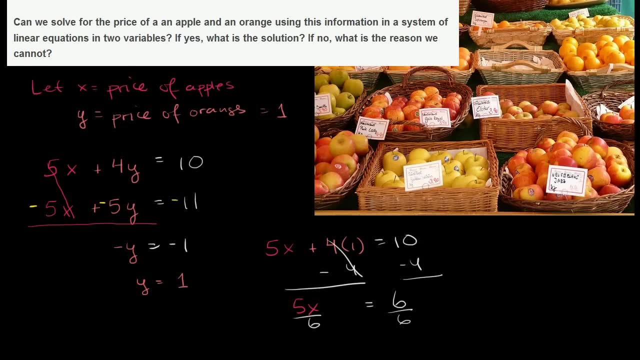 And on the right-hand side we have 10 minus 4, which is equal to 6.. And we can just divide both sides by 6 now in order to solve for x, And so we can divide both sides by 5 in order to solve for x. 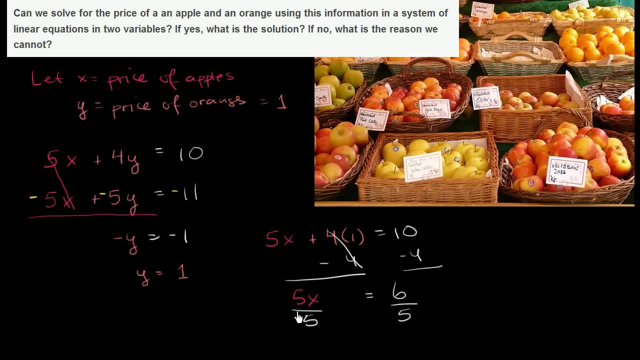 My brain isn't. it's late in the day, Brain isn't working. Dividing by 6 wouldn't have done anything. We would have gotten 5,, 6x. We just want to get an x here. So dividing both sides by 5, we get x is equal to 6 fifths. 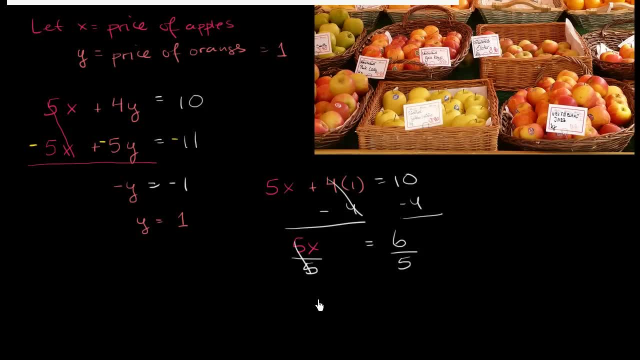 dollars. Or you could say that x is equal to 6 fifths, which is the same thing as 1, and 1 fifth, which is the same thing as $1.20.. So it's $1 per orange and $1.20 per apple. 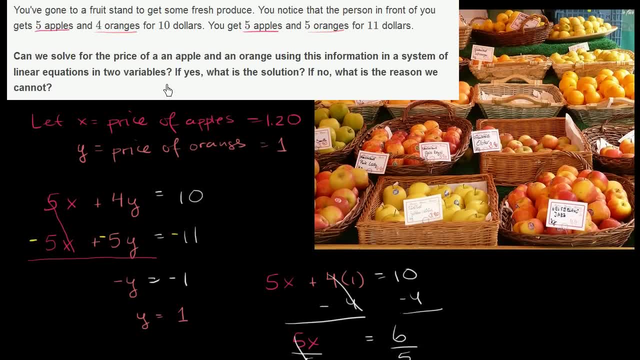 So we absolutely could figure out the prices of apples and oranges using the information given. 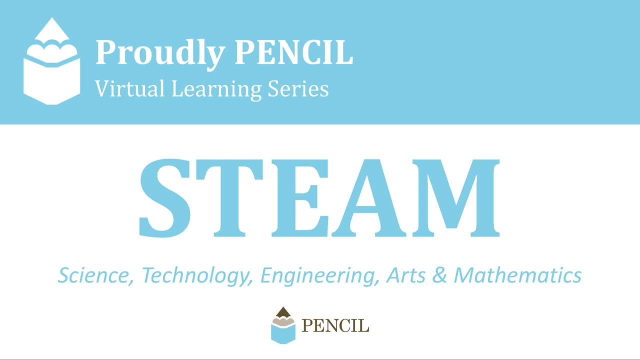 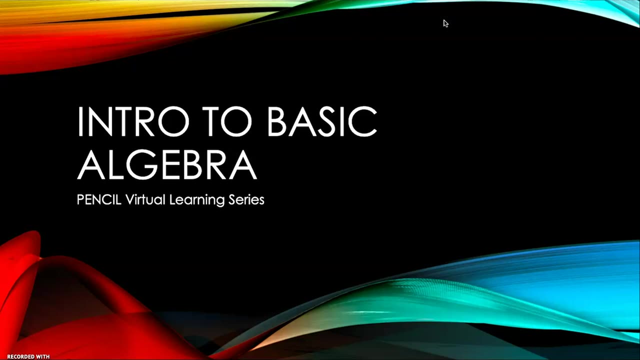 Hello everybody. my name is Elijah Osmoda and I am a pencil partner working on their virtual learning series through Hands on Nashville. Today I will be teaching you the basics of algebra. Math may seem scary and even useless to some, but I believe everyone can grasp.